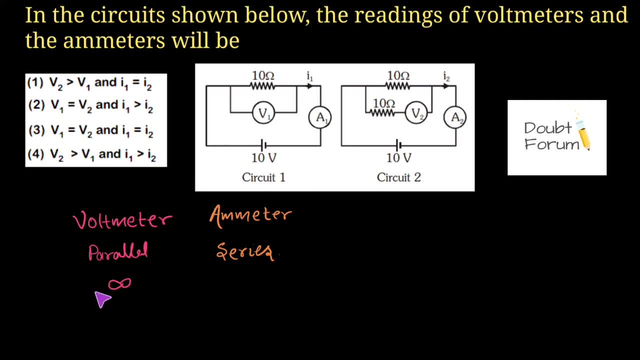 resistance would be having a value of infinite. So its internal resistance for practical voltmeter is very high, whereas for ideal the internal resistance of the voltmeter is infinite. Similarly, the internal resistance of the emitter is very low. And if we say that the emitter is ideal in 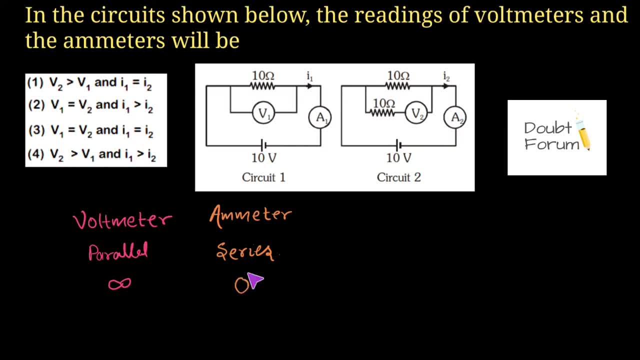 nature, its value should be zero. So these are the points which we have to keep in mind before we solve this question. So, coming to the question, in the question it is not mentioned that whether the voltmeters and emitters connected in these circuits are ideal or practical. So as long as 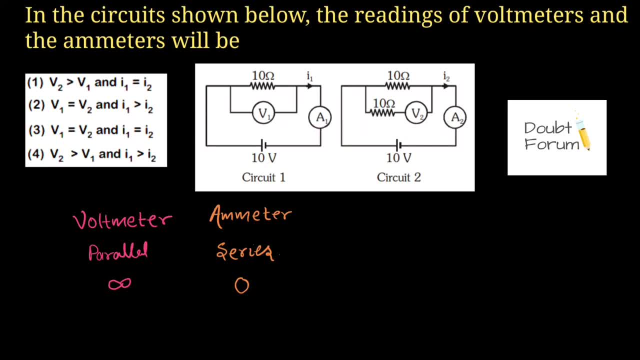 it is not mentioned and the internal resistance of the instruments are not given. we always consider that the instruments connected here are ideal in nature. So as long as the voltmeters are ideal in nature, so its internal resistance should be infinite. Similarly, if the emitters are ideal in nature, its internal resistance should be zero. So for 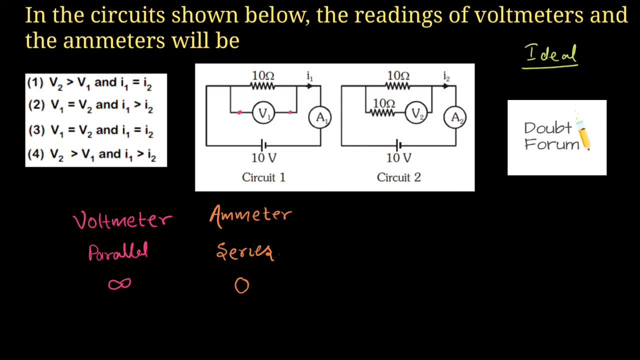 first case, if we assume that this voltmeter is ideal in nature, it means the internal resistance of this voltmeter should be infinite, And infinite means that this point A and B will behave like an open circuit. When this point A and point B is behaving like an open circuit, 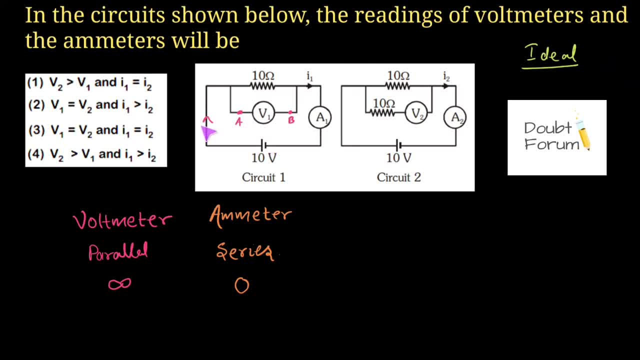 what will happen? Suppose a certain current is flowing from this voltage source, So this current would pass through this 10 ohm resistance. It will not go through this branch AB because this voltmeter is ideal in nature and it is having an infinite internal resistance Due to infinite. 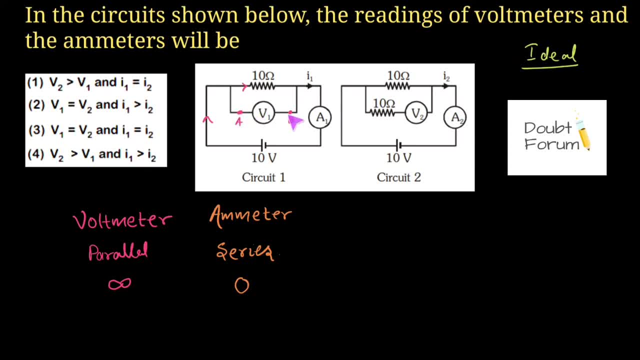 internal resistance, no current would flow from this branch AB. The next thing is this emitter. This emitter is ideal in nature. It means the internal resistance of this emitter is zero. And when the internal resistance of this emitter is zero, it will not go through this branch AB. So 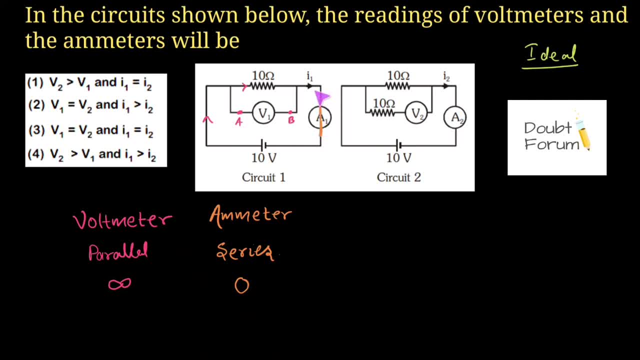 it will not create any hurdles in the flow of current. So the same amount of current would also flow from this emitter. So for circuit 1, if we want to calculate the value of current for circuit 1, we are assuming that the value of current is I1 and the value of voltage is V1. 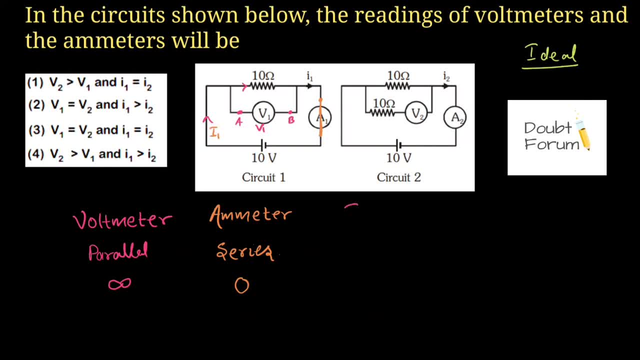 And if you want to find out the value of I1, so the value of I1 would be V1 divided by R equivalent. So from here, the value of V is this: 10 ohm, And R equivalent is representing the total resistance connected across this 10 volt voltage. 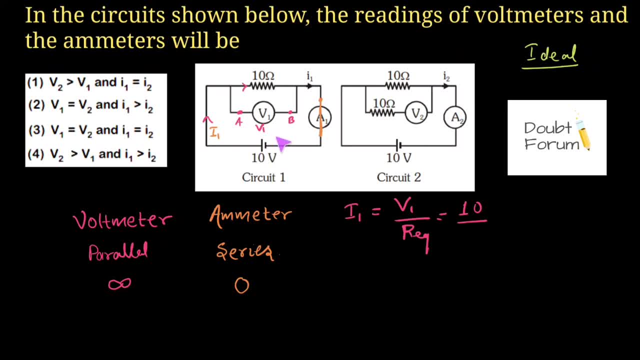 supply. So the total resistances which are connected across this 10 volt supply is this 10 ohm only Because this emitter is ideal in nature, so its resistance would be zero, While this will behave like an open circuit because it is ideal in nature. So, voltmeter, ideal voltmeter, have. 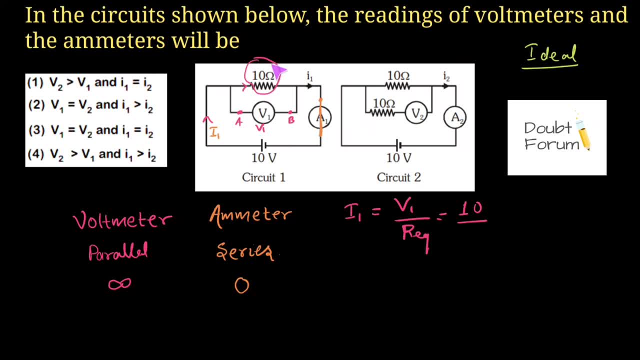 infinite internal resistance. So R equivalent would be only this 10 ohm resistance. So this would be 10 ohm. Now the value of I1 would come out to be 1 ampere And if you want to find out the reading of this V1, V1 would be representing the voltage drop. 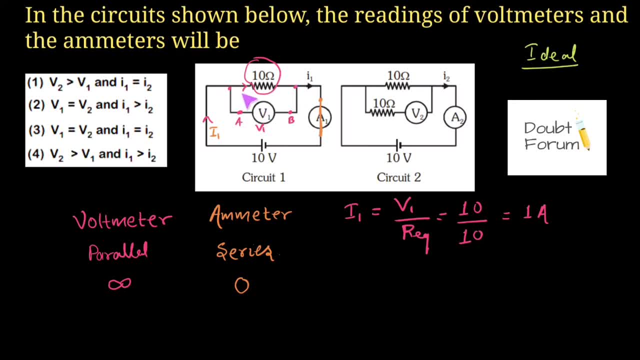 across these two terminals. Or we can say this: voltmeter would mean that the voltage drop across the element. across the element it is connected. So this V1 is connected across this 10 ohm resistor. So the voltage drop on this 10 ohm resistor will be deflected on this voltmeter. 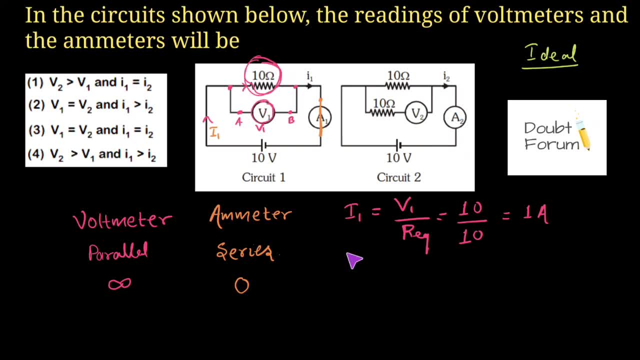 And its value would be the voltage drop across this 10 ohm V10 ohm would be I, that is, 1 ampere, into R and the value of R is 10.. So its value would come out to be 10 volt. So this would be the reading of this voltmeter. 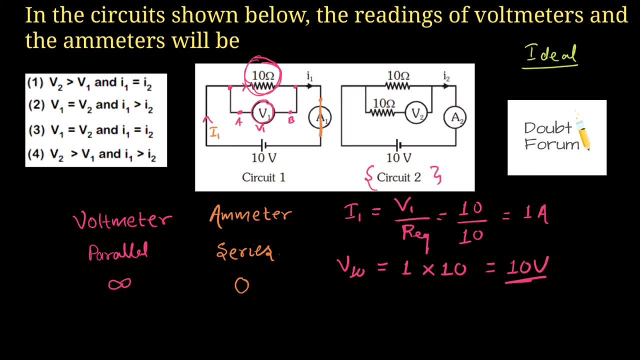 Now coming to the circuit number 2, what will happen for circuit number 2?? Suppose a current I2 is flowing in this circuit. As we have already assumed that this V2 connected here is ideal in nature, And as long as this voltmeter is ideal, it will be 10 voltmeter. So 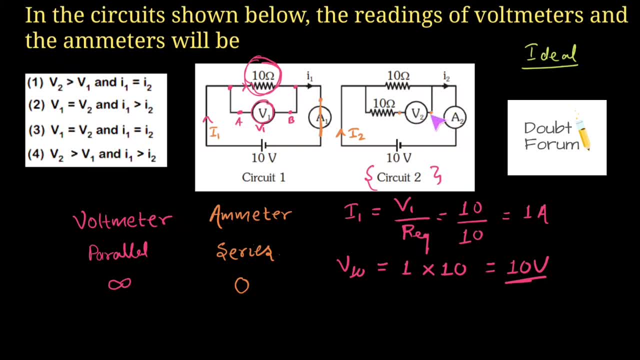 this is ideal in nature. There would be no current passing through this voltmeter And this point A and B would again behave like an open circuit. So this I2 current would only pass through this 10 ohm resistor And no current would pass through this branch Because this A and B would be acting like 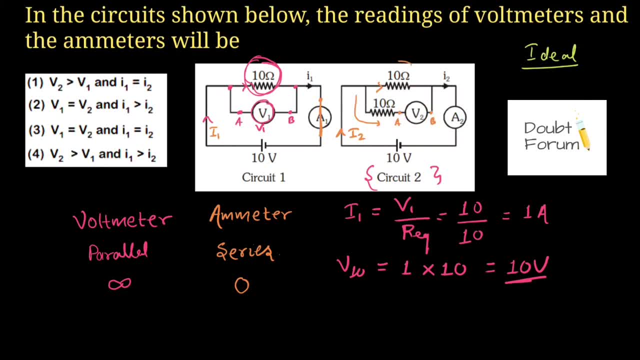 an open circuit. So whole current would pass through this 10 ohm resistor only. And here again the emitter is ideal in nature, So it will not be creating any hurdles in the flow of current. So for this circuit the value of I2,. 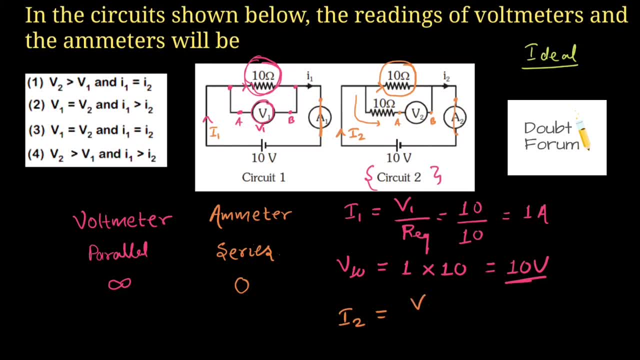 would be equal to V2.. And V2 is also equal to 10 ohm, So it would be V2 divided by R equivalent. The value of V2 is 10 volt. That is the voltage of the voltage source And the value of R equivalent.